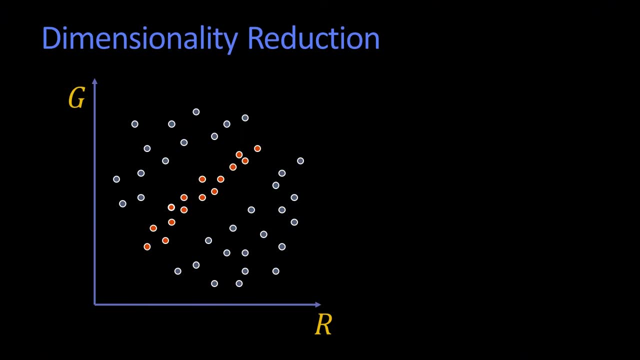 All right, if you think about these orange points, let's think about how they're distributed. okay, So they have a mean somewhere and they've got a set of eigenvectors, right. They've got a covariance matrix that describes them. 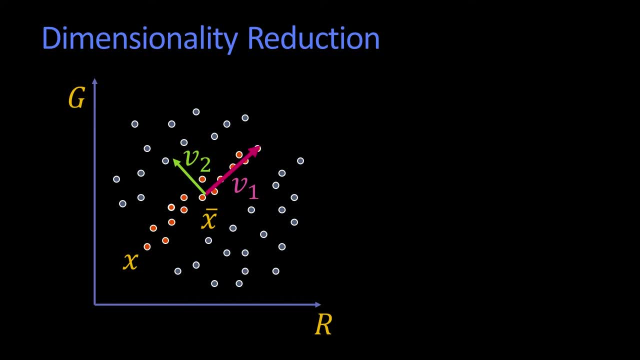 They have a axis of least inertia and then the next axis. So here you're seeing the points. the orange points are x, X bar here is supposed to be their, their mean. And then we've got the big eigenvector, v1, and then the smaller one, v2.. 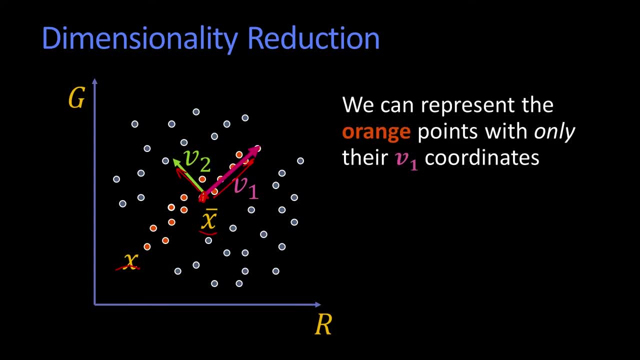 And the idea is we can represent those orange points by only their v1 coordinates plus the mean, And what that would mean is ha ha. essentially that we're going to think of all the orange points as just being on that line And all I'm going to tell you is where on the line they are. 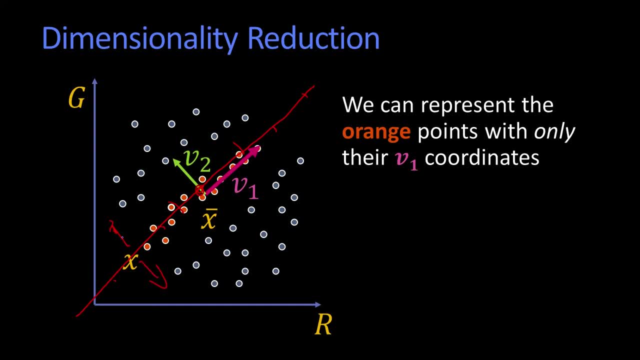 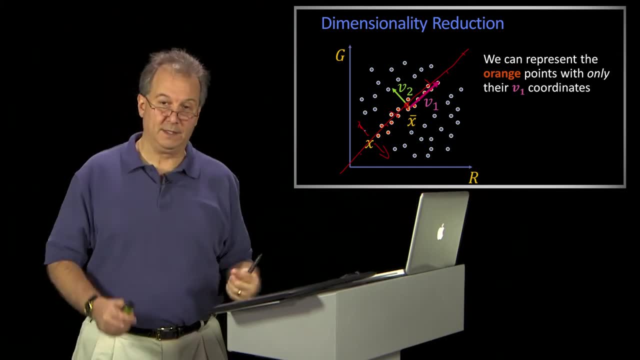 And we're going to essentially ignore the amount that they're off that line. So we've just reduced the dimensions From how many Two To how many One. Okay, that doesn't sound like that big a deal, nor is it. 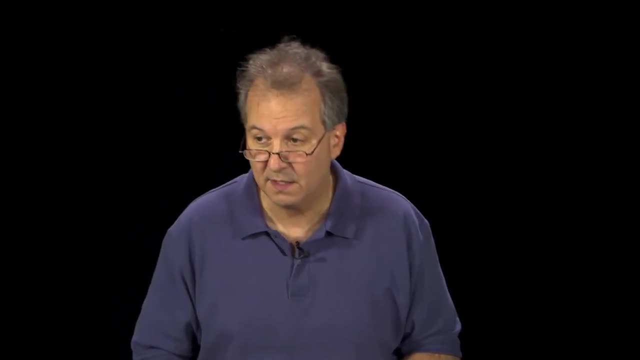 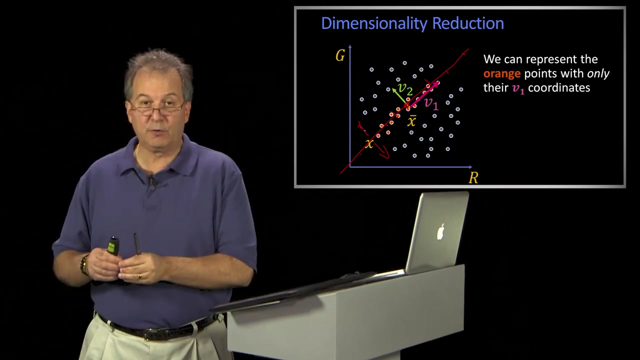 But in higher dimensions this could be a huge deal. Imagine you've got something in 10,000 dimensional space And yes, in just a minute we're going to do a 10,000 dimensional space. If you said, well, I'm going to represent them by one number, or even 30,. 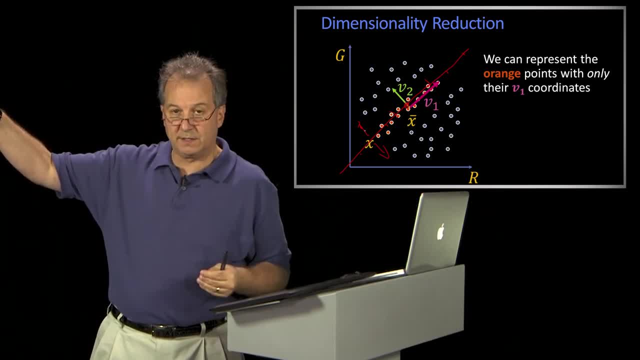 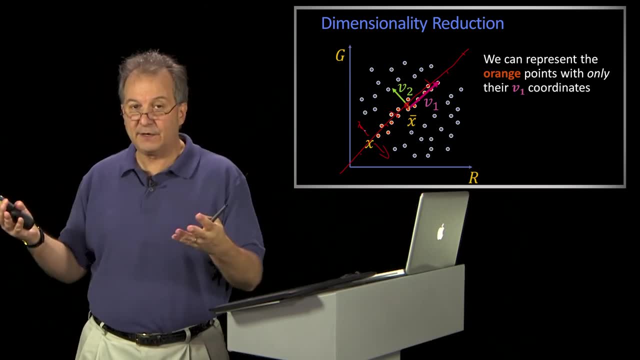 that would be a huge reduction. So if I say, well, what direction does it vary the most in- And I just give you that value, If that's good enough for what we want to do- you've reduced the description from being a lot of numbers to being a much smaller number. 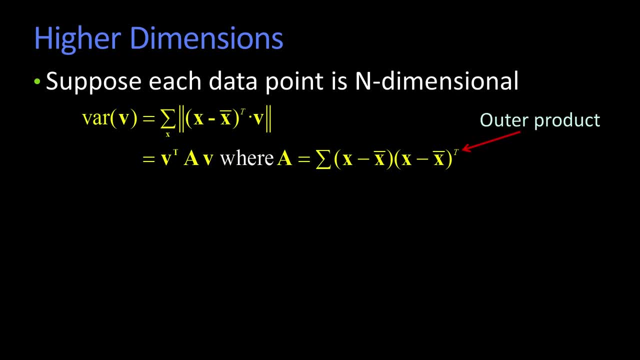 In fact, we can sort of express that here algebraically in terms of just thinking about it, whatever dimension x happens to be in. So I've got a whole bunch of data points in some n-dimensional space. What I want to know is the direction of projection and 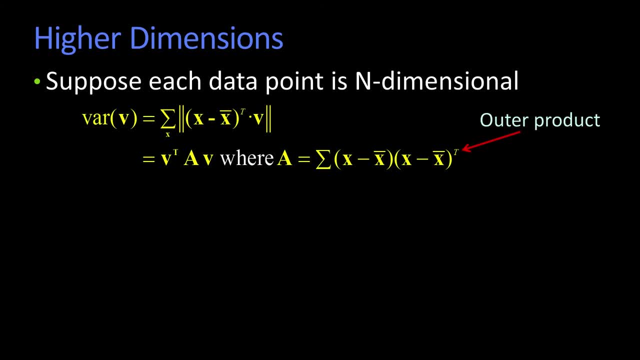 we'll say it's v. all right That if I projected those points after subtracting out the mean that I'd have the greatest amount, right, The greatest variation, And that's what that says here, right? So take x.